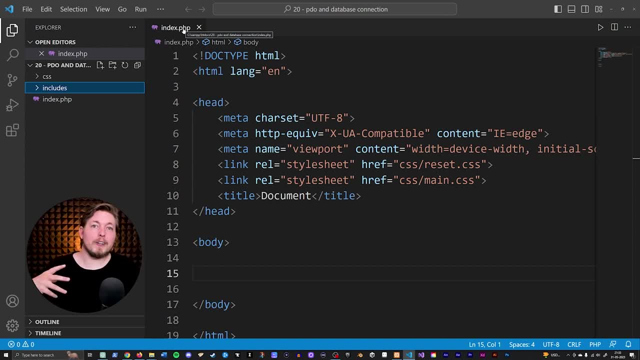 page. So the include files are just basically extra files that just run code. The first thing I'm going to do inside this folder here is create a new file. So I'm going to say I want to create which stands for DatabaseHandlerincludesphp. 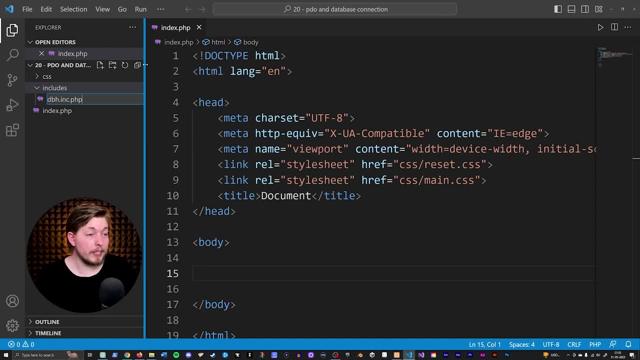 Now it's very important to point out here that it is possible to go in and name it as dbhinc, which is also a kind of file that we can use and create PHP code inside of, But this kind of file can create issues. 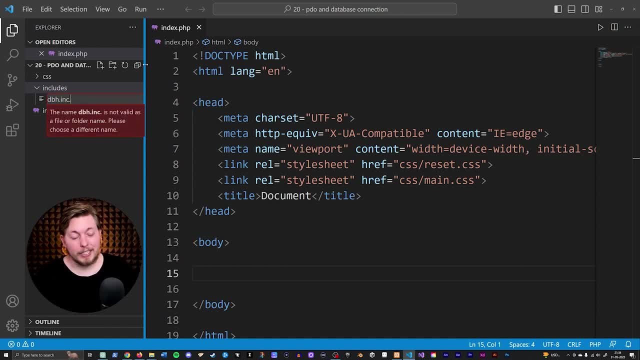 And some people, when they hear that I call it incphp, think that we are creating a inc file. That's not what we're doing here. The inc is just a naming convention, So to speak, So it doesn't really do anything. 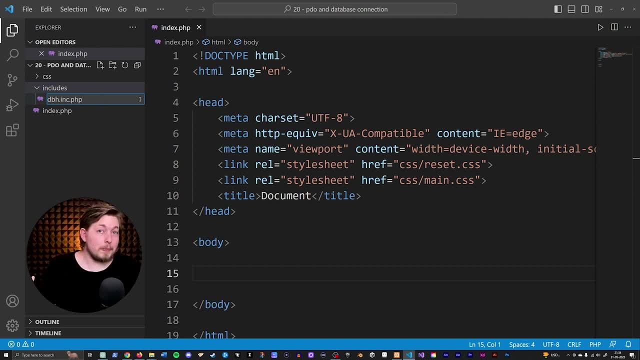 This is going to be a PHP file, So in this case, if you could call it dbhinc, or you could call it dbh-inc, or just dbh-inc if you wanted to, It's really the same thing, because it's just a name. 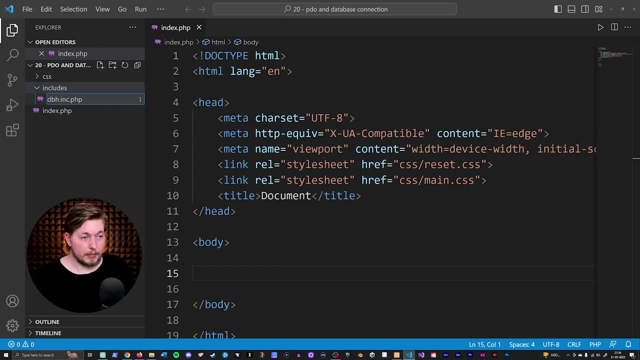 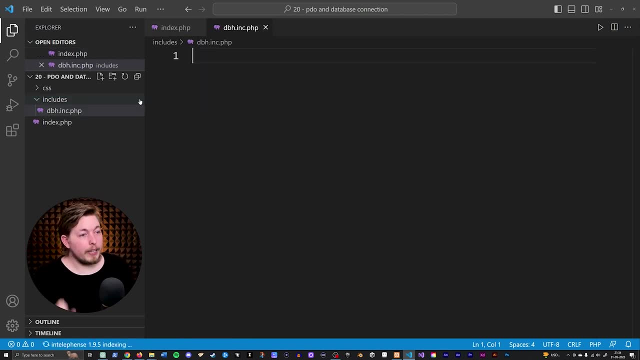 So don't get confused about the naming convention that I'm using here. It's just a way for us, as the developer, to know exactly what kind of file this is. So what I'm going to do is I'm going to name this file and create it. 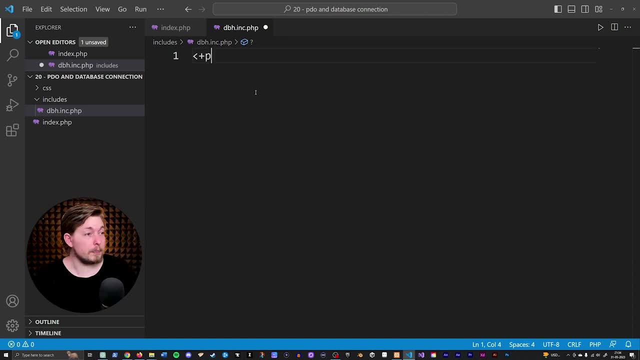 And inside this file I'm going to open up a PHP tag so we can actually create some PHP code. And it's important to point out here- because we talked about this in my syntax video at the very beginning of this course, that when we have a pure PHP file, we don't create a closing tag. 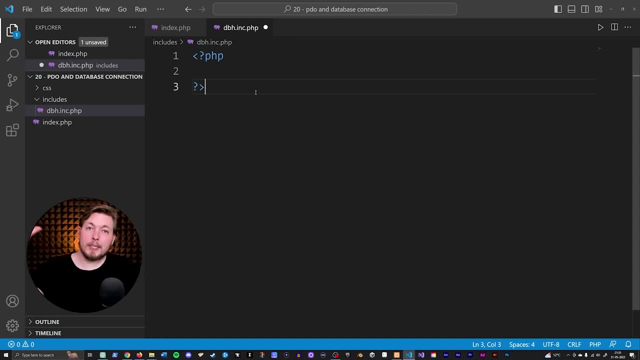 So, for example, you would create this at the end of a pair of PHP tags. We're not going to do that when it's a pure PHP file, And the reason for that is if we were to accidentally go below here and create some HTML or something just by mistake. 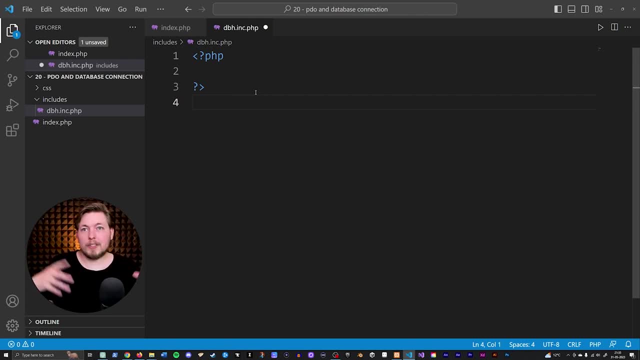 then we can create more damage than not doing that. Again, you can always go back and watch that episode at the beginning of the course if you want to know more about this, but we're just not going to put it in here, So going in here. what we can do is we can start off by saying: 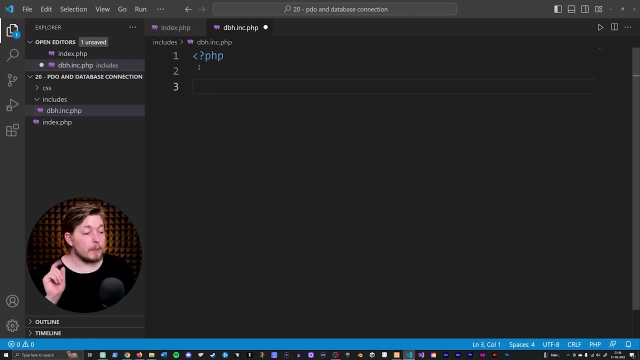 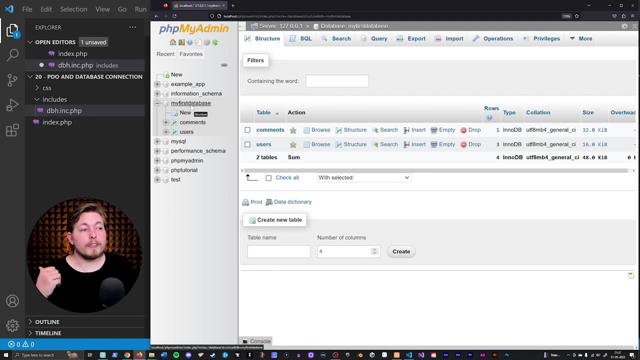 that we want to include some information about our database. We did, of course, create a database in the past couple of episodes, So if we were to go in here, you can see that I created a database called My First Database, And inside this database we also created a couple of tables. 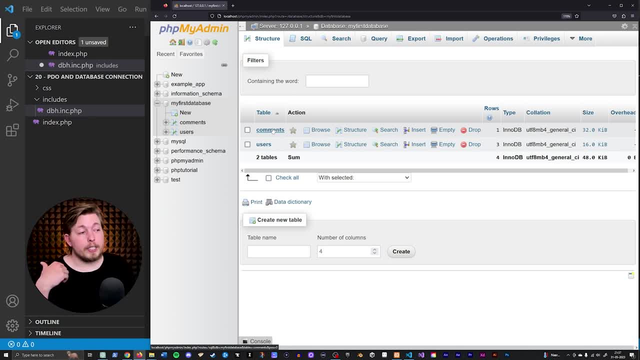 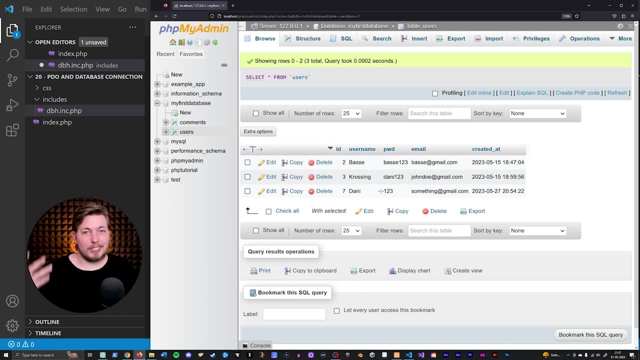 that could actually have some sort of information inside of it. So we have a, So we have a, We have a comments table and we have a users table. We actually do have some users, just because we learned how to insert and update and delete data and that kind of thing. 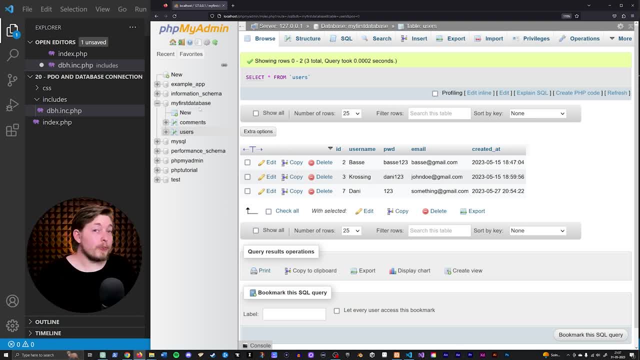 So we have some stuff in. here is what I'm trying to say. All we have to know for now is that we have a database called My First Database, because we do have this phpMyAdmin hooked up to our server, So when we do actually need to connect to our database, 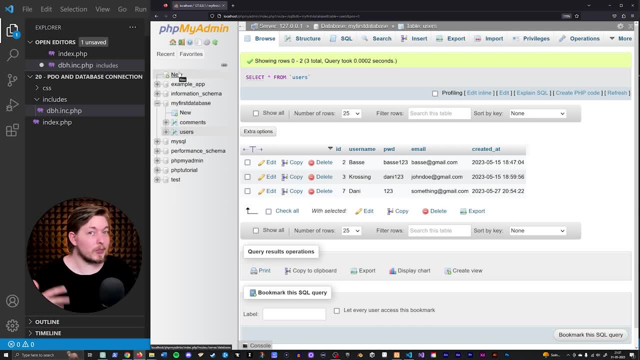 we do need to tell it which one of all these databases we're trying to connect to, because it is possible to use more than just PHP. It is possible to use just one database inside a website. You can use multiple if you want to, And there is arguments for doing that. you know, for different reasons. 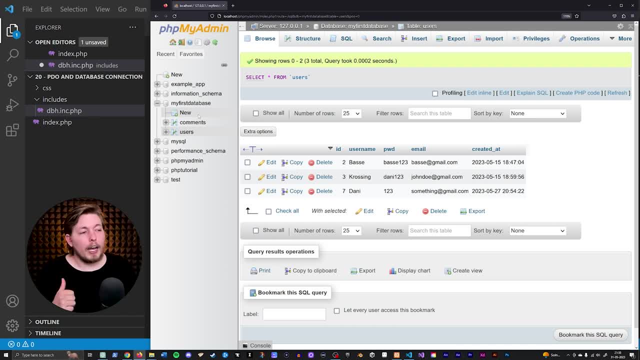 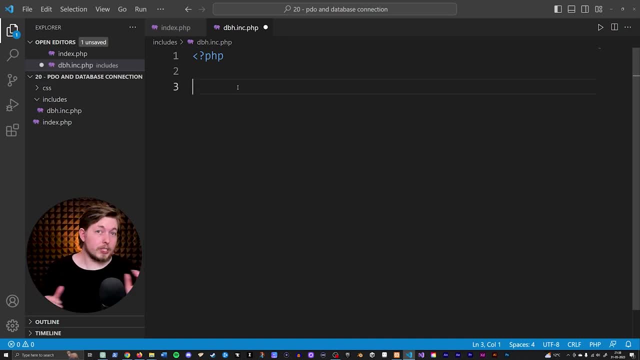 But for most websites you're just going to have one database for everything, So remember the name: My First Database. So, going back inside our file here and I'm going to create a DSN, which stands for Data Source Name, which is us telling our server what kind of database driver we're trying to use. 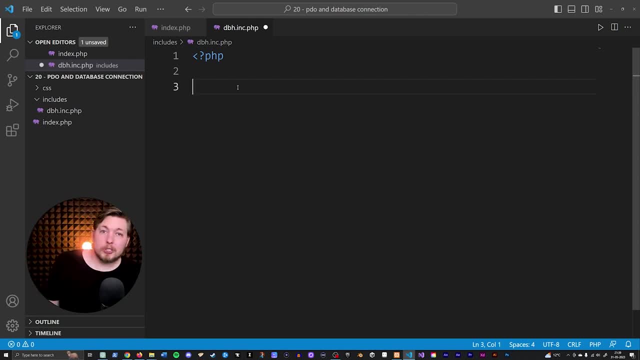 and what is the database name? what is the host that we're trying to connect to? In this case, it's going to be localhost, So we need to give it a little bit of information about this database we're trying to connect to. 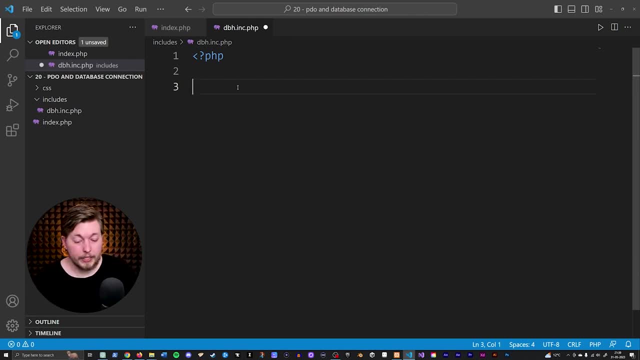 So in our case, we're using a MySQL database, So we're going to create a variable. I'm going to call this one DSN And I'm going to set it equal to a string, And inside of this string here I'm going to say that I want to connect to a MySQL database driver. 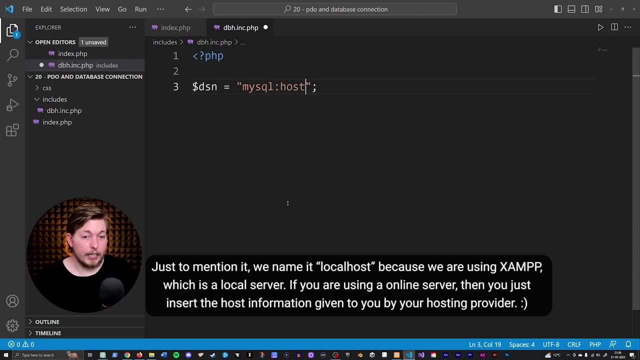 Then I want to tell it what kind of host I'm trying to connect to here. In this case it's going to be localhost, So I'm going to say equal to localhost semicolon, And then I want to tell it what kind of host I'm trying to connect to here. 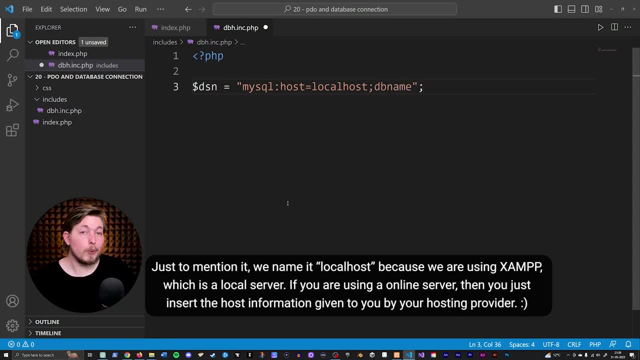 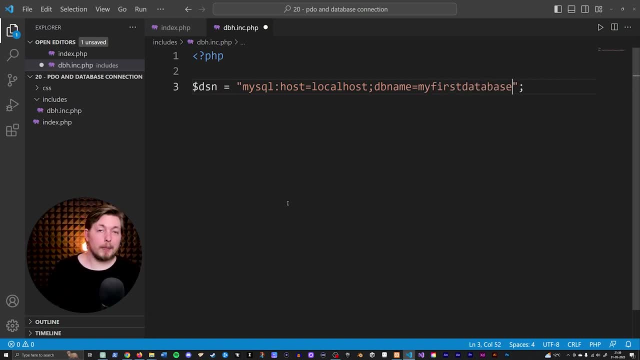 So I'm going to tell it the database name which in this case here we did already just go in and check. In my case it's called MyFirstDatabase And again, if you call this something else in the past couple of episodes, 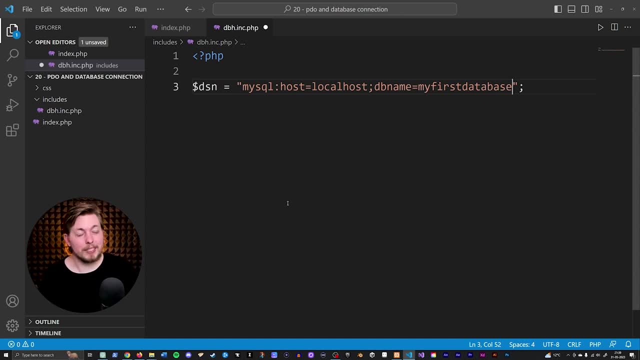 you do need to change this So it matches whatever you called your database. So you basically just go in and change the information here depending on what database you're trying to connect to. So underneath here I need to give it two more pieces of information. 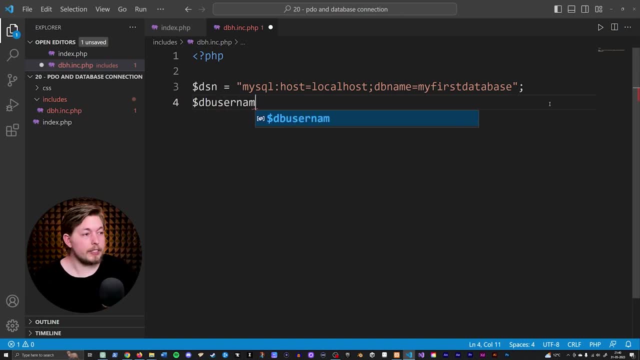 I want to give it a database username, So we're going to say dbusername, And this one is going to be my database And this one is going to be my database, And this one is going to be my database And this one is going to be equal to root. 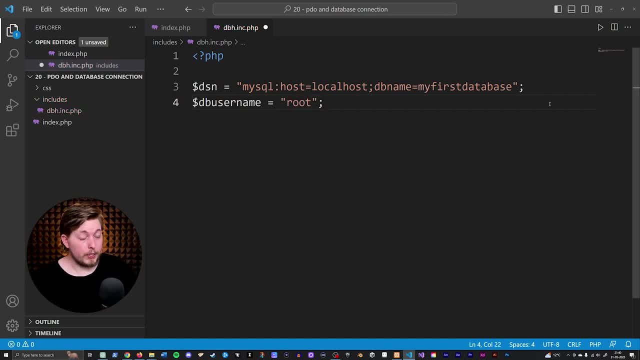 And I do want to explain this in just a second, but let's go ahead and create the next one as well. So I'm going to create a database password, And this one is going to be empty, in my case, here Password. There we go. 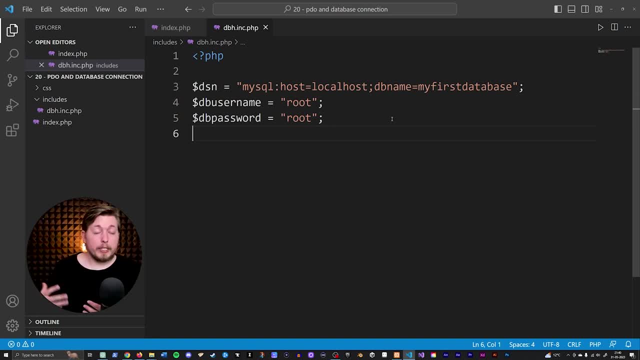 So, basically, when we have a database, we do also have a username and a password in order to connect to our database, which makes sense. So, in my case, because I'm using my XAMPP software and I have not gone in and actually changed this- 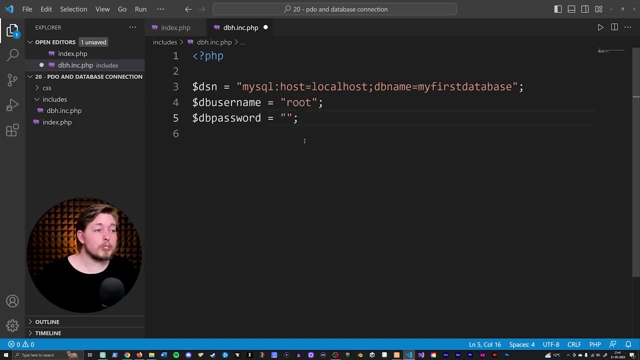 the default username and password is going to be root and then no password. I do want to point something out here, though, because if you're using a Mac computer, you may need to go inside your password and write root, Because I did experience 12 years ago. 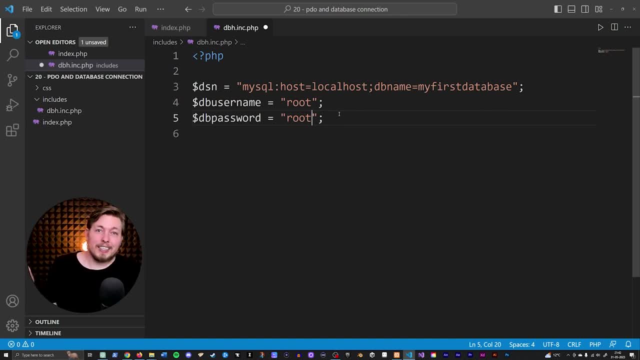 when I was studying my web development bachelor's degree, that people who were using Mac computers and using XAMPP did actually need to include root in both places, because XAMPP is a little bit different on Mac than it is on Windows when it comes to root. 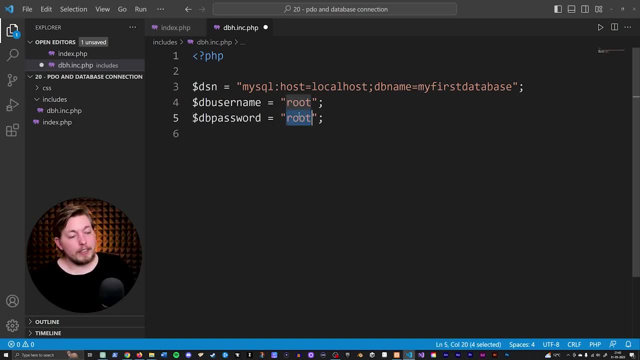 So if you're sitting on Mac and doing this right here doesn't work for you, try writing root both places and see if that works for you, Or just Google how to change your password and username for your database. Again, there's a couple of different options here. 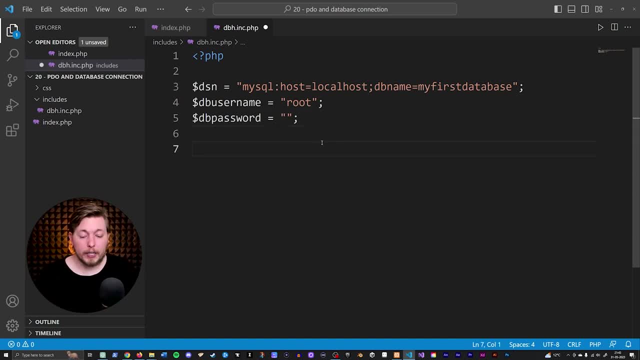 We're just going to stick with this information for now, And then I actually want to go down and run a try-catch block So we can actually see we get a pop-up here and it looks like this. So basically we have a try-catch block. 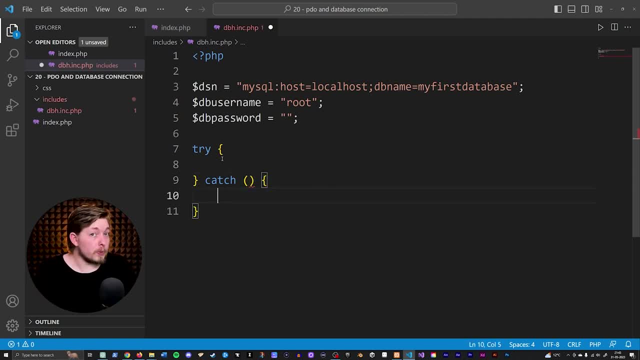 which means that we are basically running a block of code and if an error occurs, then I can do something else by catching the error and then doing something with the error message. That's basically what a try-catch is, And you'll see this very often inside PHP. 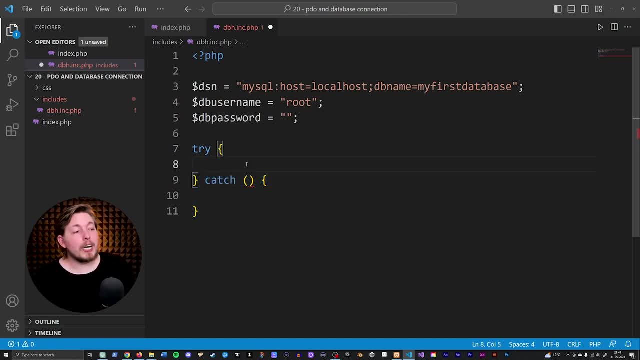 because a try-catch block is very useful. So what I'm going to do inside my try is: I'm going to say that I want to run a PDO connection, and we didn't actually talk about this yet, because when it comes to connecting to databases, 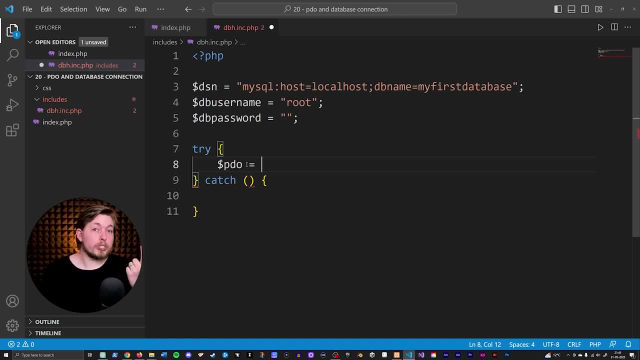 we have three different ways we can do it. We have what is called a MySQL connection, which is very bad and you should never use that because it's obsolete, And they actually came up with a new way to connect to a database which is called MySQL. I. 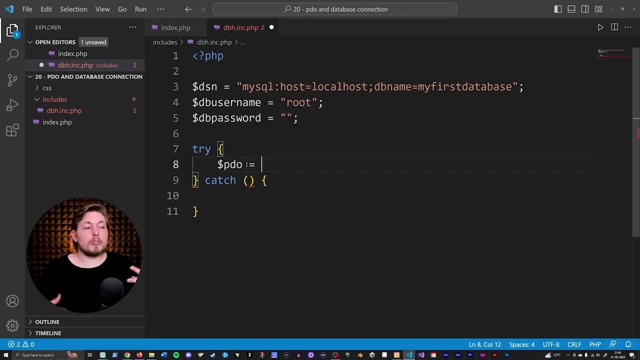 which stands for improved. This basically goes in and does extra SQL injection prevention. So don't use MySQL, because there is some security things that is just not very good. But now let's not talk more about ways that you cannot connect to a database, because we have talked about that now. 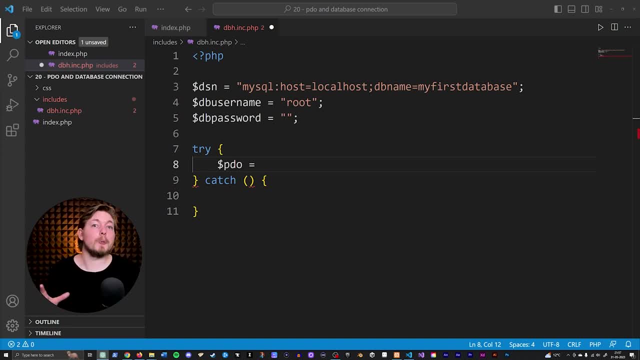 But what you can do is you can connect to a database using MySQL I, or we can also use the third method, which is called PDO. Now, PDO stands for PHP Data Objects, which is basically another way for us to connect to a database. that is a little bit more flexible. 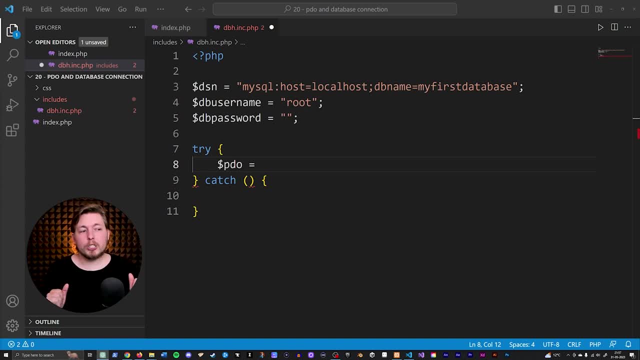 when it comes to different types of databases out there- MySQL. I is very good when it comes to MySQL databases, but if you plan to connect to other types of databases, for example SQLite or something, then you can use something like PDO. It has also been a thing in the past lessons of mine. 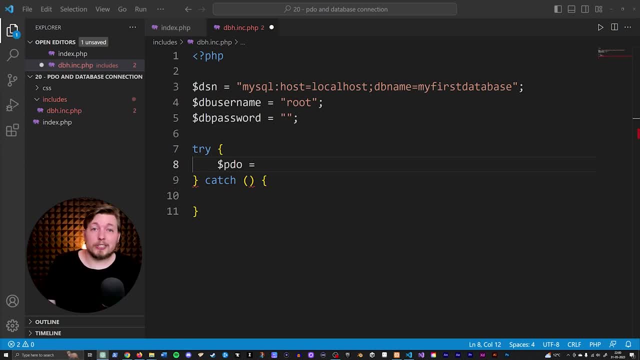 that people do request that I use PDO. So we are just going to stick to using PDO, since that is going to be the one that people lean more towards, because it is more flexible. But for people who are curious about what exactly the difference is when it comes to the actual programming, 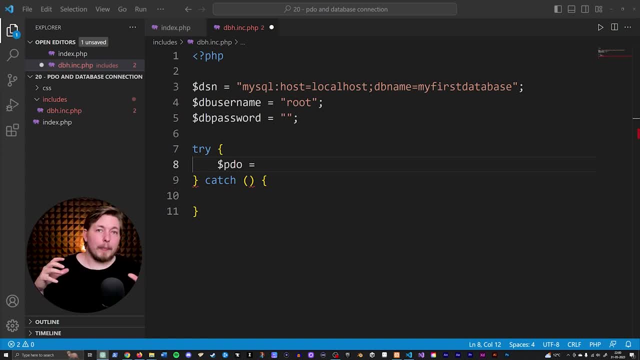 when it comes to MySQL I and PDO, it's basically just the methods that change a little bit when you start programming it. If you are curious about MySQL I, you are more than welcome to look it up, but we are going to be using PDO in these lessons here. 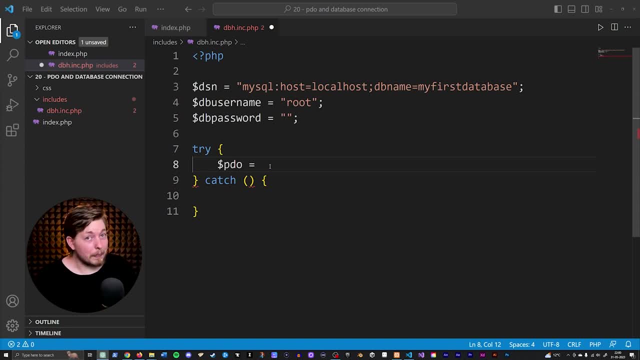 So, having ranted a little bit about different ways to connect to a database, we are now going to create a PDO connection. So PHP data objects is a way for us to create a database object when we want to connect to a database. So basically, we turn a connection into an object. 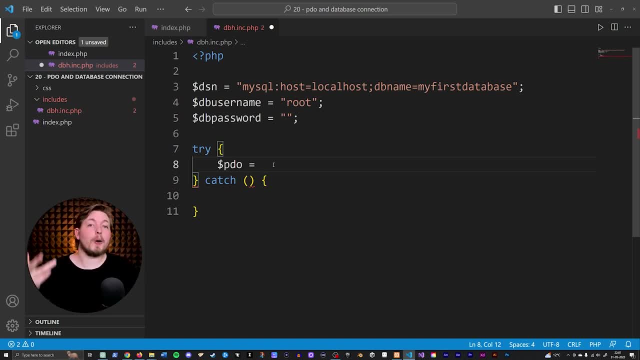 that we can use inside our PHP code and just refer to that object whenever we want to connect to a database. So what we are going to do is we are going to have a variable called PDO. I'm going to go inside of it and create a new PDO object. 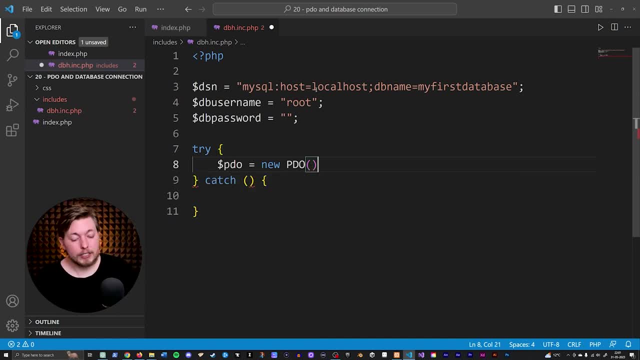 So we are going to say new PDO And what this basically does is that it instantiates a PDO object off of an existing class inside our PHP language that is going to create this connection based on a couple of parameters. So, for example, what is the database driver going to be? 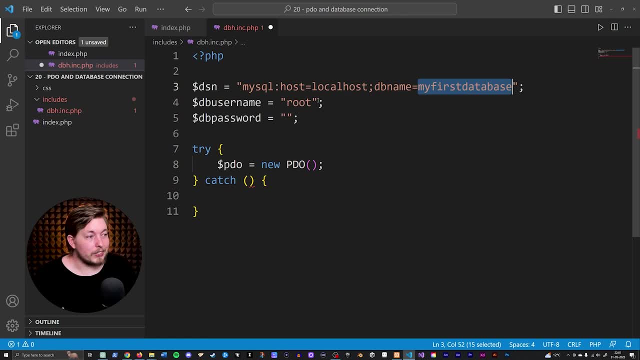 What is the host going to be, What is the database name we are connecting to, What is the username, What is the password? And then it's going to create a database connection object that we can use. So, going inside this PDO, I'm going to give it a couple of parameters. 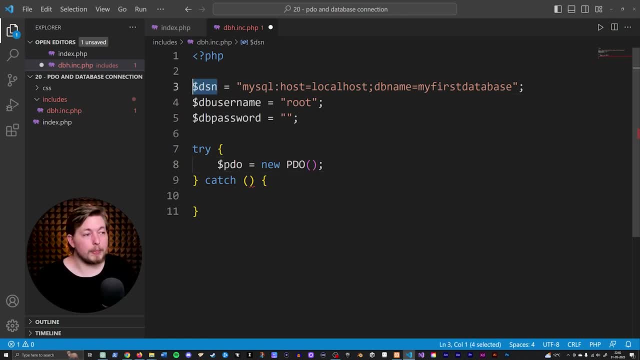 The first one is going to be the DSN which we just created up here, So we have all of this information. Then I'm going to give it the username, So we are going to say DB username, And then I'm going to give it the database password. 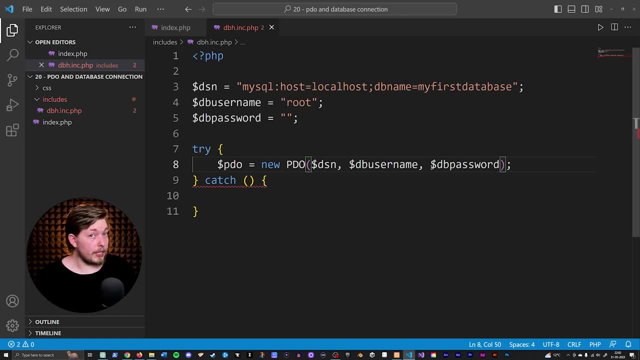 So doing this here we now have a database object And, just to mention it here, we could technically just take this one line of code and do this right here, And that would actually be enough to connect to our database, if all the information is correct every single time. 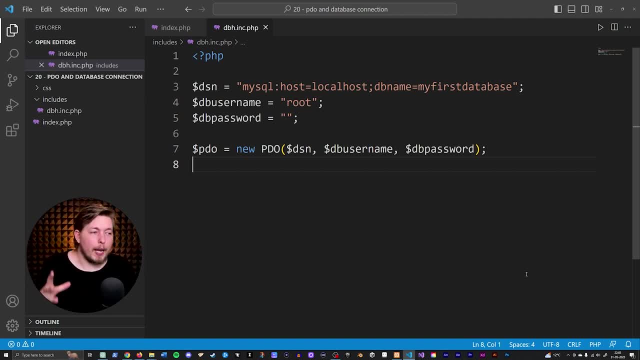 But we do want to have some sort of error handlers. if an error happens, then we want to be able to grab that error message and show it inside our website. So even though this is like the pure bare bone enough to connect to a database, it is a good idea to run this. try cats block here. 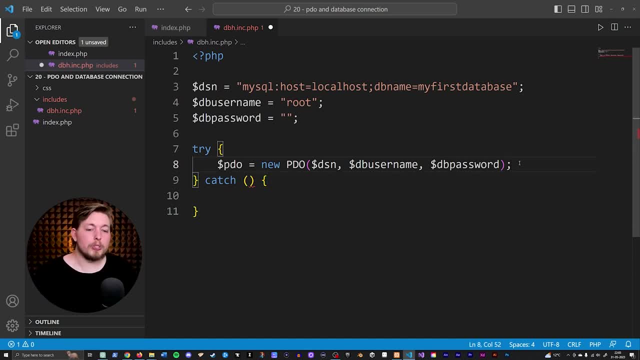 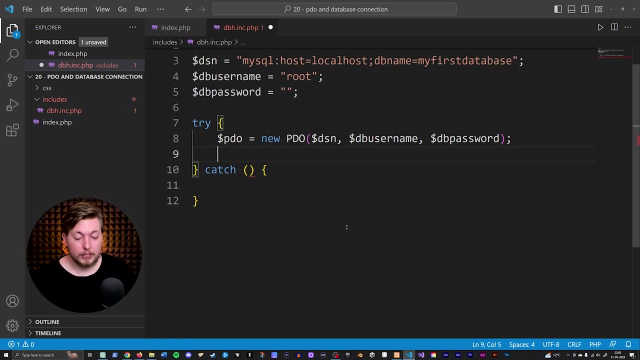 to get any sort of potential errors. So what I want to do is I want to set a couple of attributes inside this object that we created here. We can do that by going in and say we want to grab this PDO variable or object that we just created here. 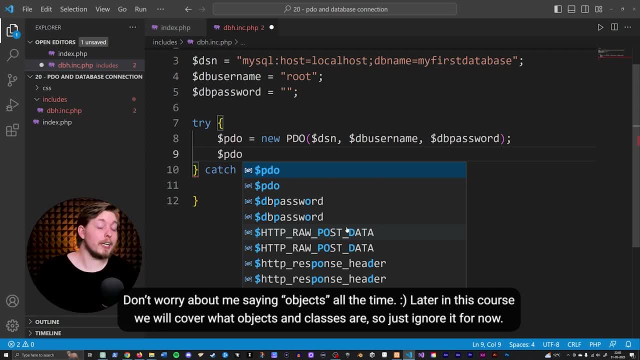 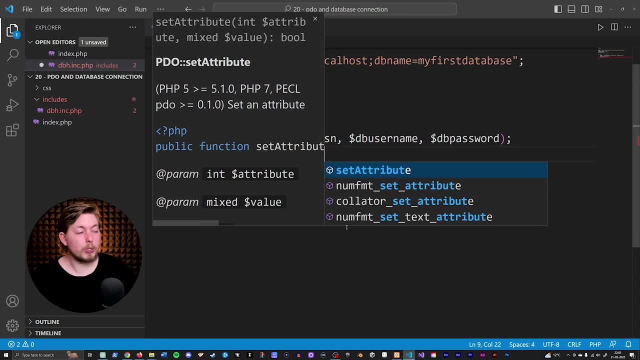 because now it's no longer a variable, it is actually an object, And I want to point to an existing method inside this object, called setAttribute, which is going to allow for us to change a couple of attributes about this particular object that we just created. 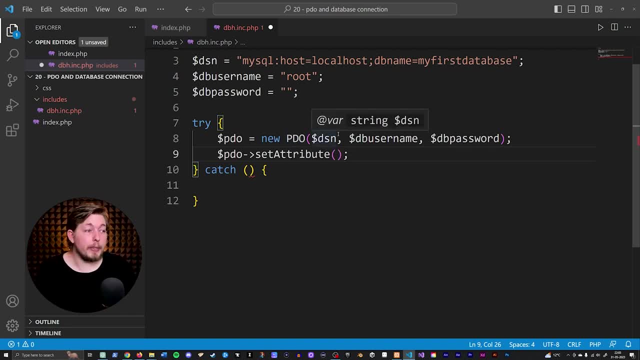 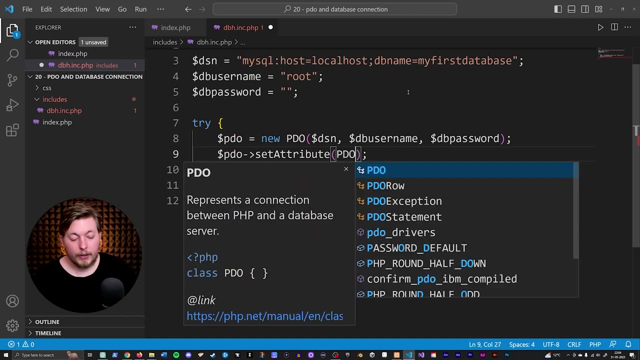 For example, how do we want to handle error messages that we may run into when we try to connect to our database? So inside the parameters here I can say I want to grab a specific attribute. So in this case it's going to be PDO, colon, colon, ATTR, underscore error mode. 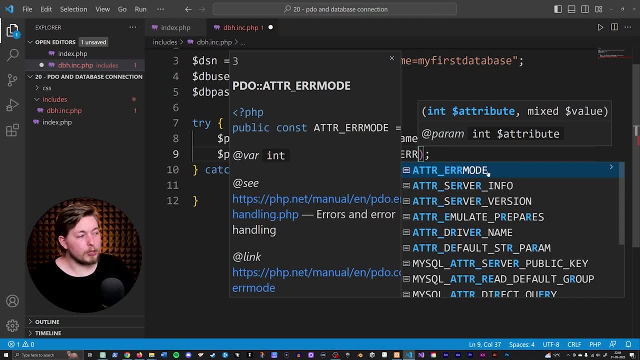 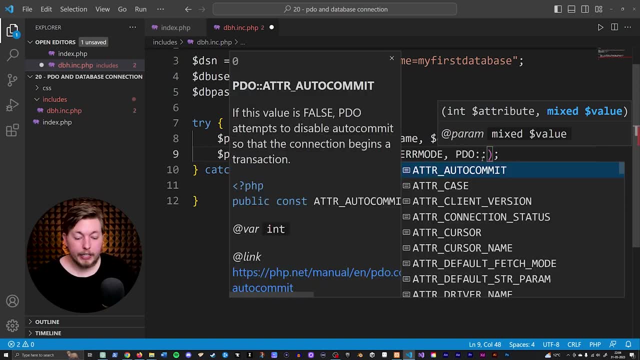 so E-R-R-M-O-D-E- you can actually see it pops up over here. So we're going to grab the error mode and then we're going to say we want to set it to a PDO colon. colon E-R-R-M-O-D-E underscore exception. 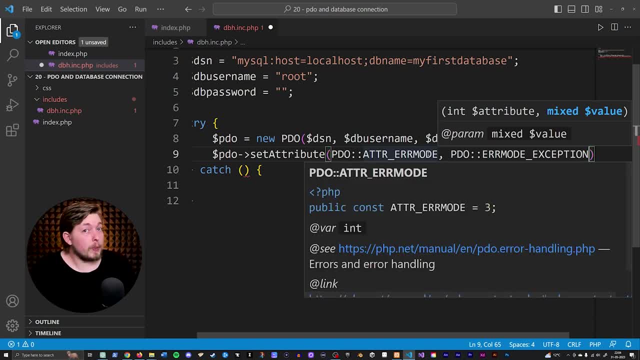 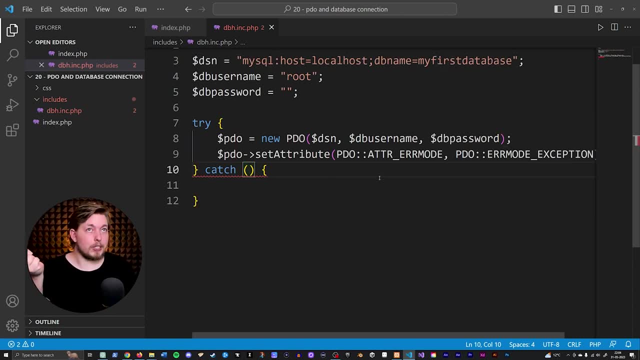 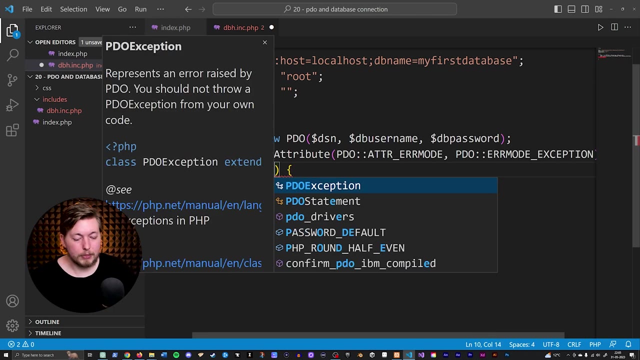 So right now we are saying that if we get an error then we want to throw an exception, which means that we can go down inside our cats, block down here and actually grab that exception, which is information about this error here. So what I can do is I can say I want to catch my PDO exception. 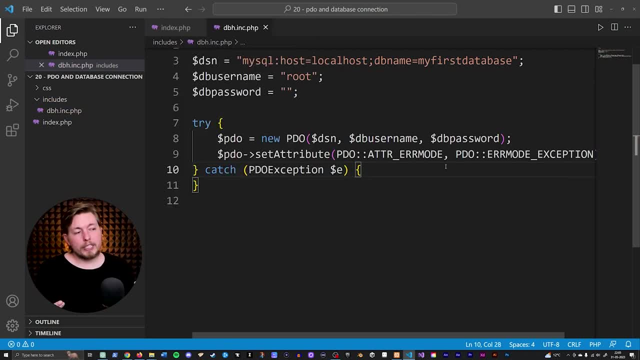 and I want to name this one variable E. So we're basically just saying that this is a PDO exception type which is going to be named as variable E, which is a placeholder that we can refer to inside the curly bracket, so if an error message happens, 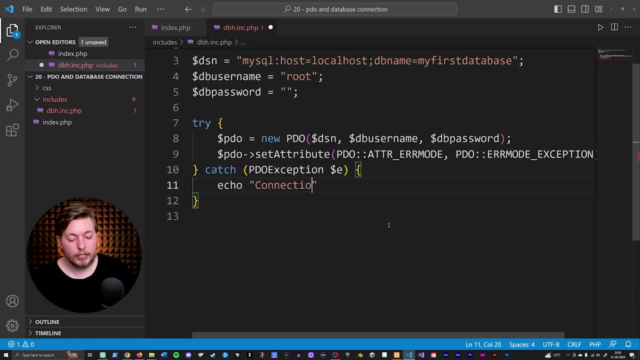 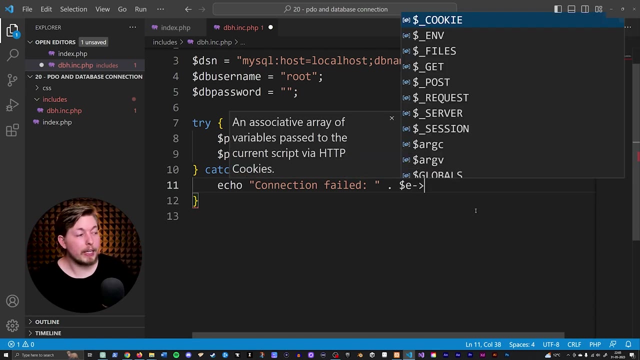 then I want to go in and echo out a message- connection failed, colon space- and then I want to concatenate a error message. so right now we are grabbing the exception by referring to variable E. so I want to go after here and paste that in and say: I want to run a method called 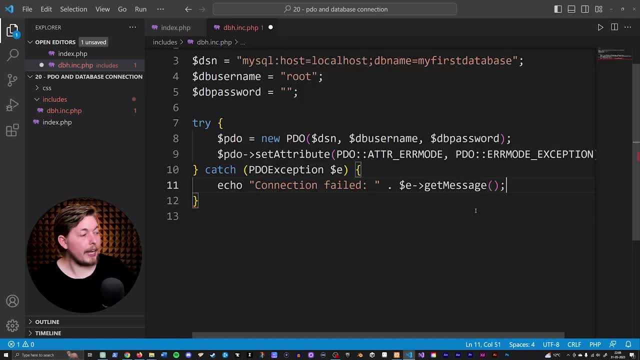 get message, parentheses and semicolon. so right now we're getting the exception, which is the error that may be thrown, and then we want to grab the actual error message and echo that out inside the browser. so if we don't connect correctly to a database, then just go ahead and throw an exception here. 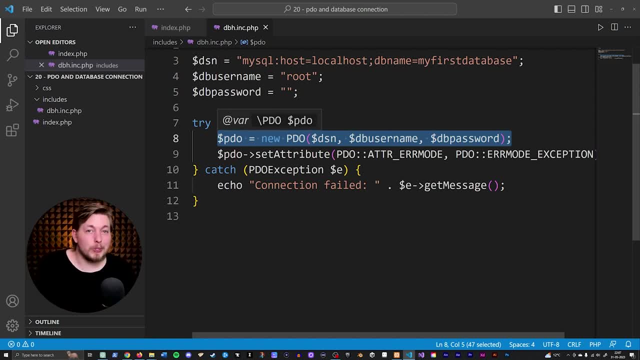 but, like I said, this one line of code here is actually the one line that we use in order to actually connect to our database. so all this other stuff down here is error handling and throwing error messages inside the screen if the connection fails, that kind of thing. 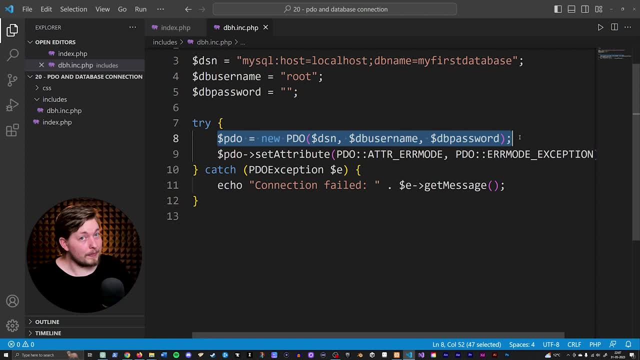 so for now, just know that this line here is the important one. So now that we have this, we can actually go in and actually do stuff inside our code. so if I wanted to select data from a database or if I want to insert data inside my database, 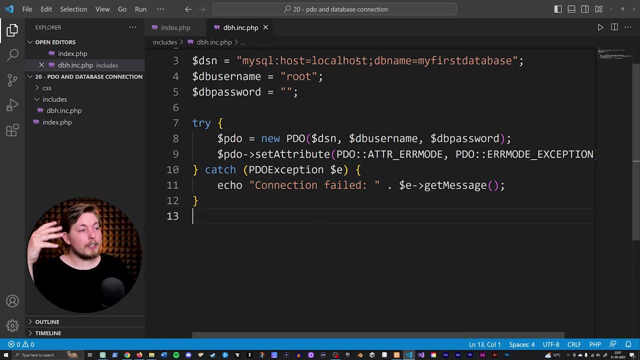 I can do that by simply running this one connection here and actually query something into my database using PHP code, and we haven't talked about how to do that yet, but that is something we're going to talk about in the next upcoming lessons. so for now, we learned how to connect to our database.